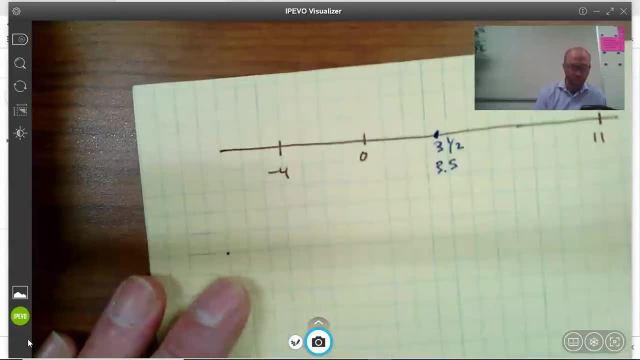 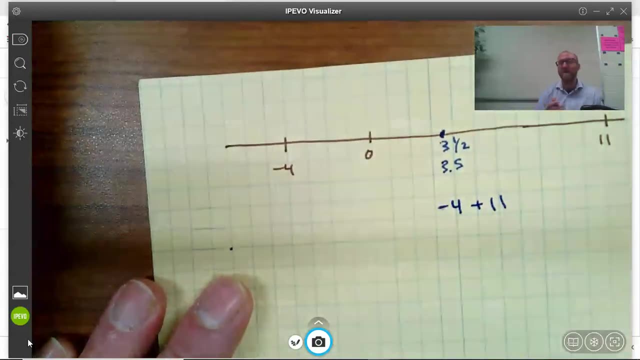 So it's the number that's halfway in between the two. So here, for example, if I wanted to find the average, I would go negative 4 plus 11.. So you just add together the two numbers and then you divide by the number of numbers, which is 2.. 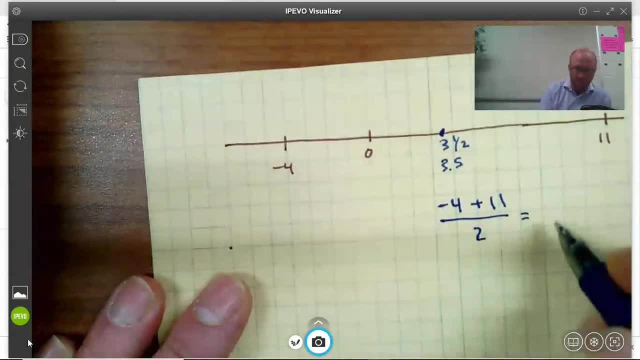 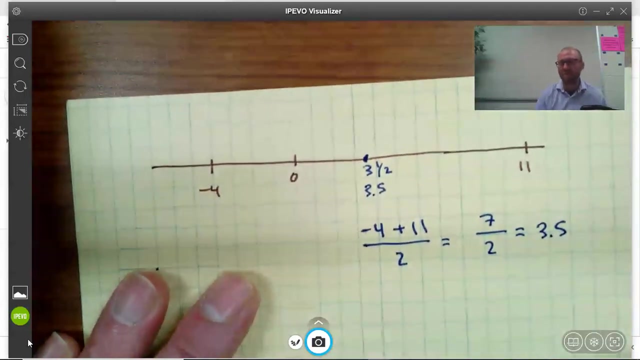 Divided by 2.. See negative: 4 plus 11 is- let's see 11 minus 4,- 7, over 2.. And that equals 7 over 2 is 3.5.. You're punching your calculator and check. 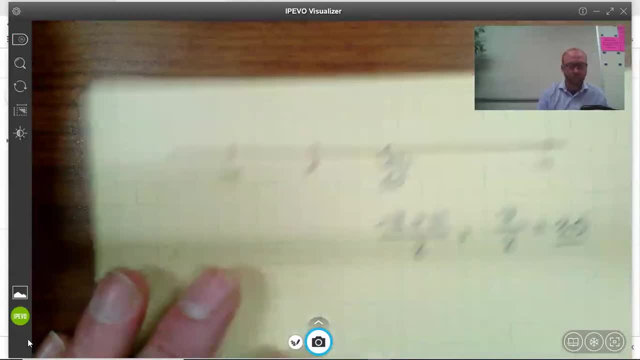 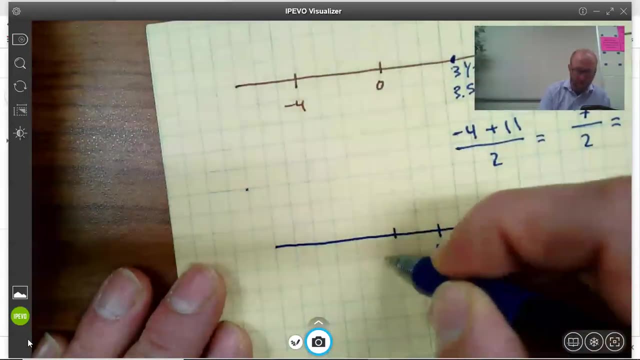 So the halfway point is 3.5.. I can do that with any other pair of numbers. Let's see. Let's find something else. I've got- I don't know- Negative 2. And 1,, 2,, 3,, 4,, 5.. 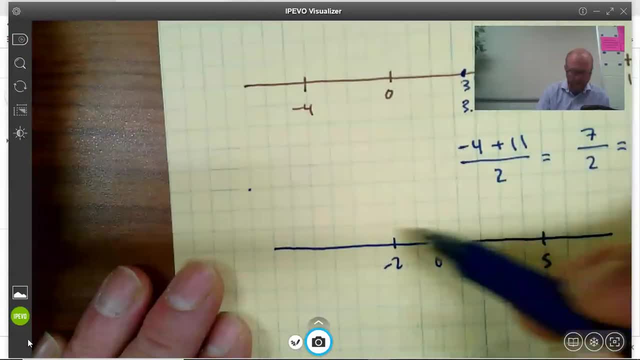 Negative: 2 and 5.. So the halfway point. they are 7 apart. So it's 1,, 2,, 3, 4, 5, 6, 7 apart. So 3.5, 1,, 2,, 3, and a half, which is 1.5 in the middle. 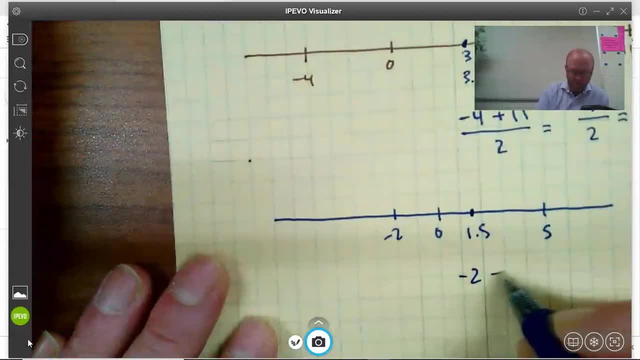 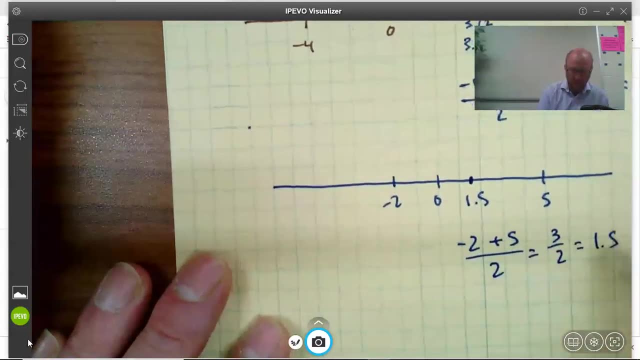 1,, 2, 3, and a half. But if I use that same formula, negative 2 plus 5 over 2.. Negative 2 and 5 is 3 over 2, which is 1.5.. 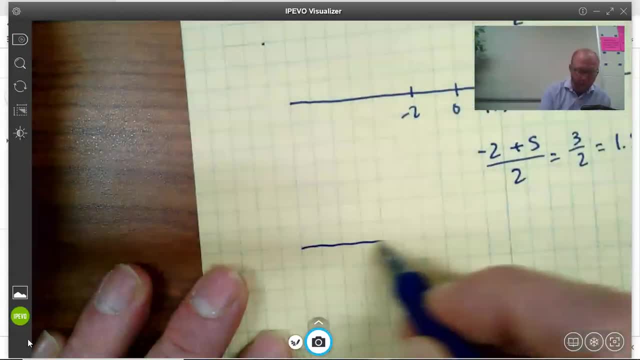 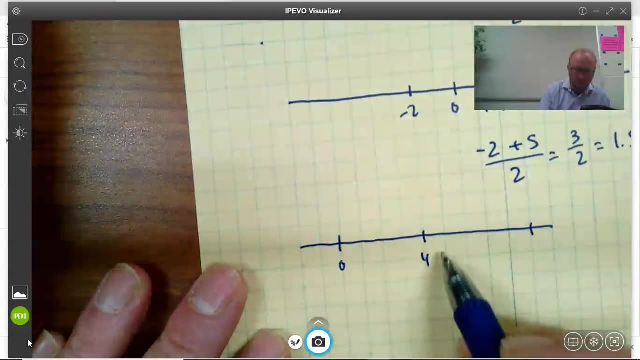 And they don't have to be, you know, two negative numbers, Maybe it's a couple of positive numbers, So maybe I have these two here: 1, 2, 3, 4, 5, 6,, 7,, 8, or 9.. 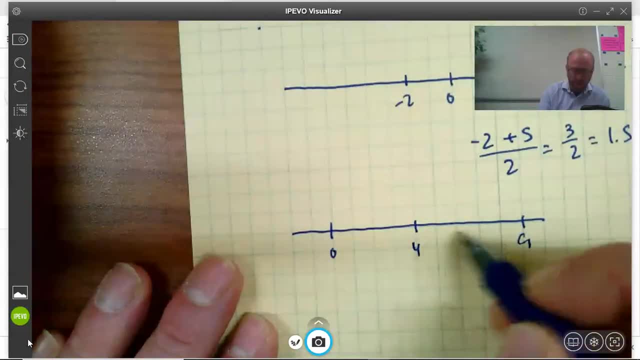 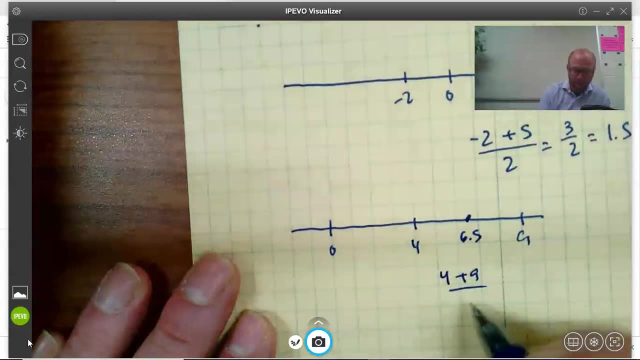 It's a halfway point. See, they're five spaces apart. So 2.5, 1,, 2, and a half, That's 6.5.. But using our formula, add together the 2 and divide by 2.. 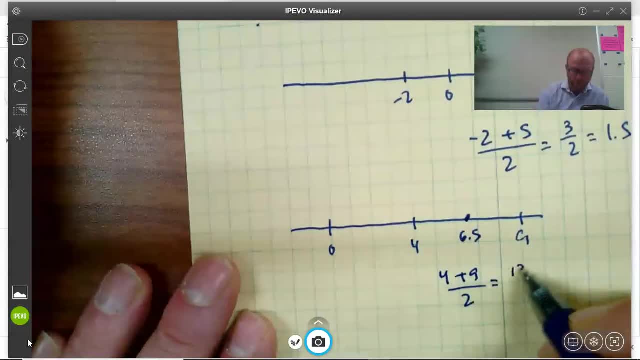 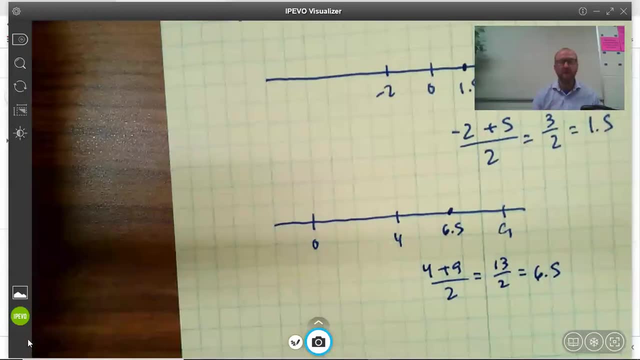 Taking the average of the two numbers, 4 plus 9 is 13.. Over 2 and 13 divided by 2 is 6.5. So if you want to find a number that is exactly halfway between two other numbers, you just add them together and divide by 2..